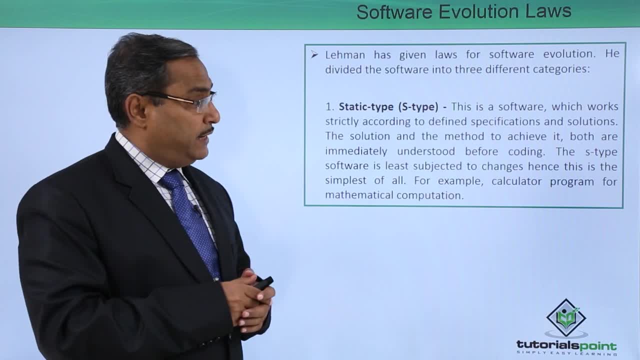 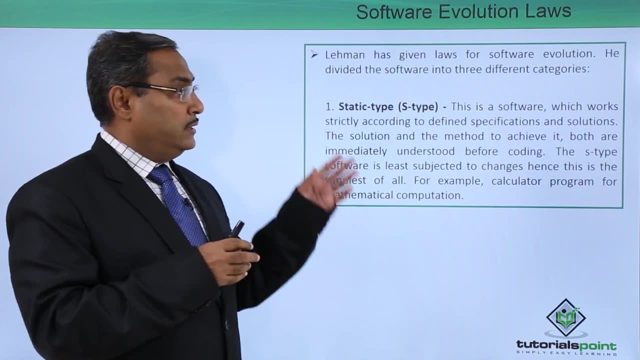 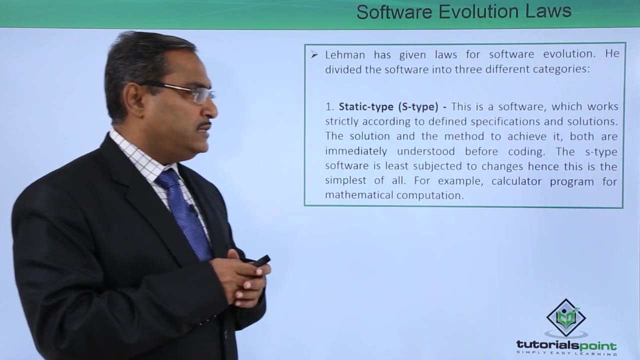 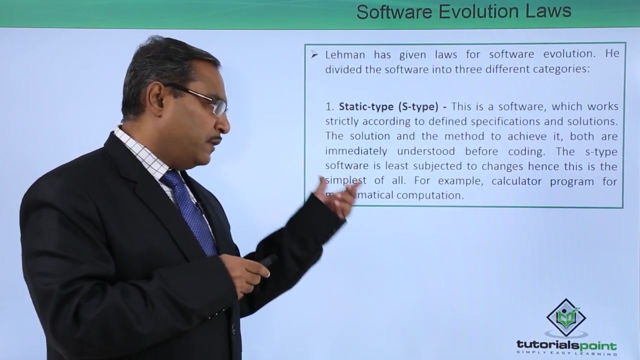 strictly according to the predefined specifications and solutions. So before developing, before starting or initiating with the development process, the software respective specifications and solutions will be pre-known to us. This solution and the method to achieve it both are immediately understood before starting the coding operation. The S-type software is least subjected. 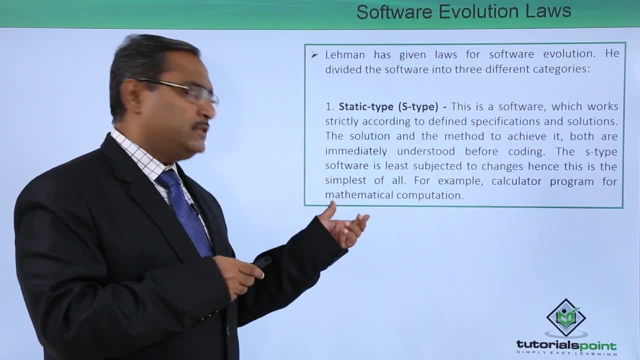 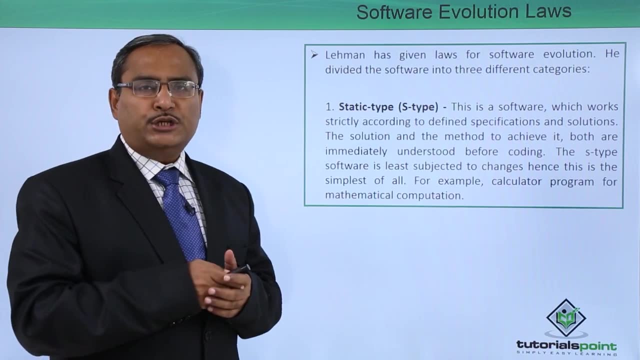 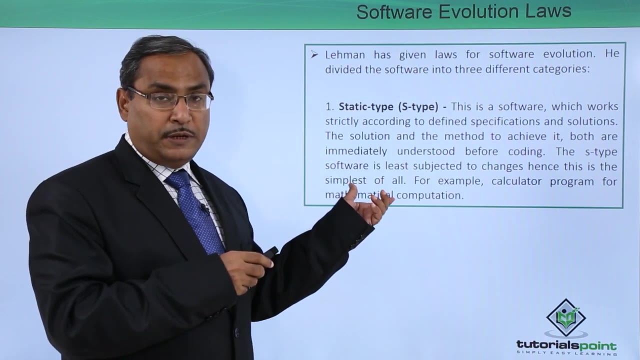 to changes. Hence, this is the simplest of all the software categories, For example calculator program for mathematical computation. we can consider So here, all these requirements are pre-known to us and we also know the respective method to achieve it. So before starting the 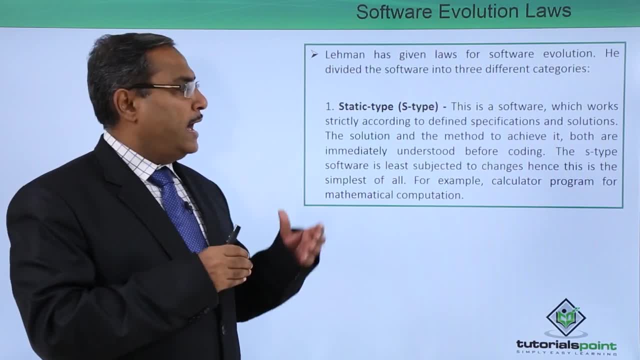 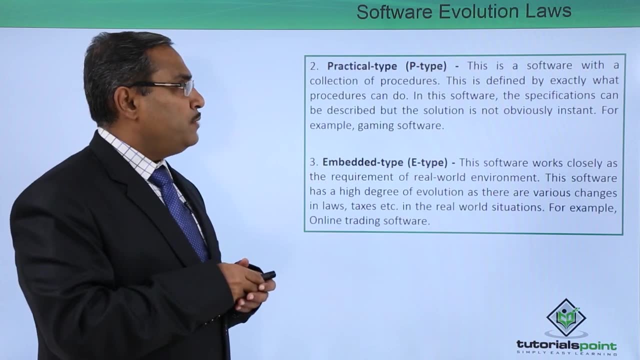 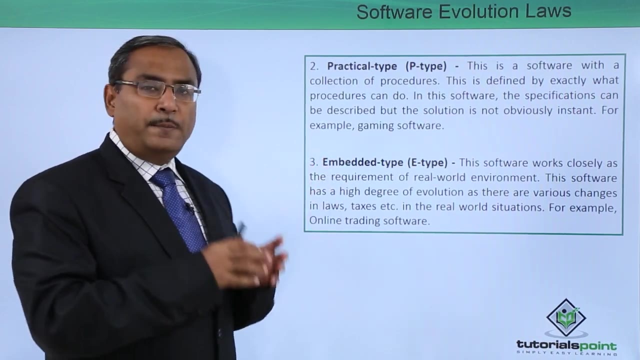 coding process. this information will be prior to us and then we shall start this coding process. and this is the simplest software category. Next one: we are going for the practical type. In short, it will be known as the P-type. This is the software with a collection of procedures, and this is defined by exactly. 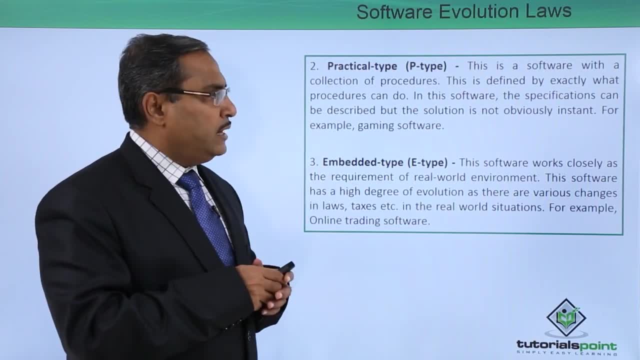 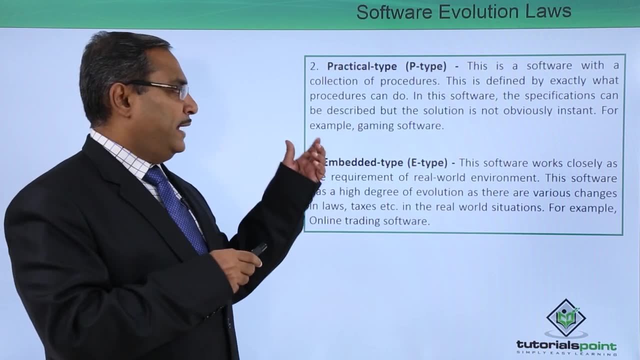 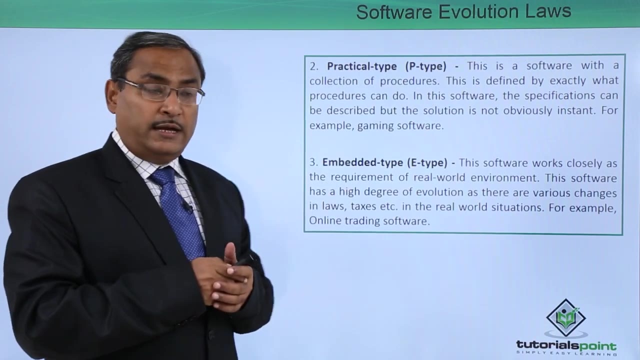 what procedures can do In this software. the specifications be described, but the solution is not obviously instant. For example, the gaming software. If you consider the gaming software, it will be falling under this practical type. Here we are, knowing that we are having certain procedures. we are having and these procedures- 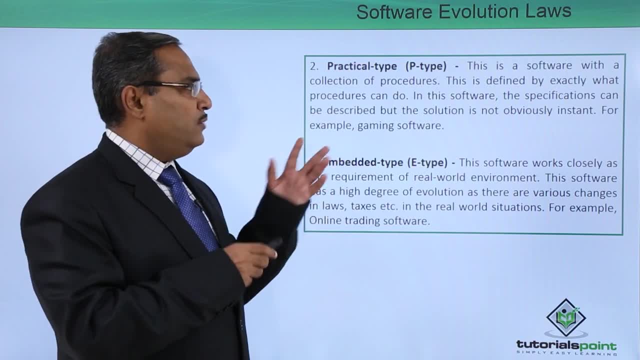 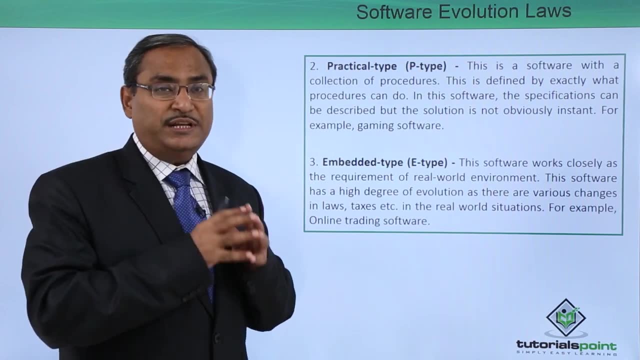 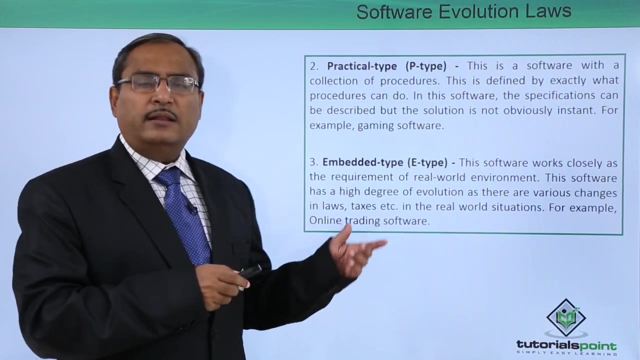 you know what we are doing, and this is defined by exactly what procedures can do In the software. the specifications can be described here, but the solution is not instant. but in case of S-type, the solution was pre-known to us. Next one, the last one, is the embedded type. in short, it will be called as E-type. This 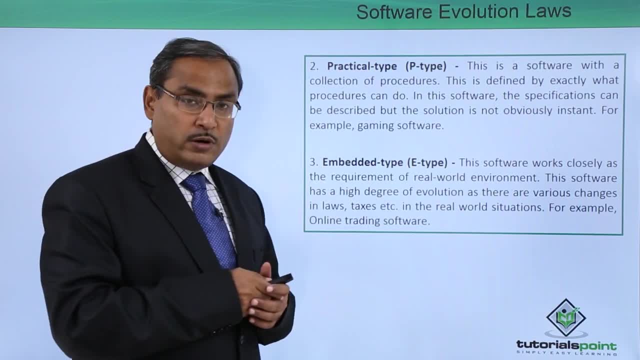 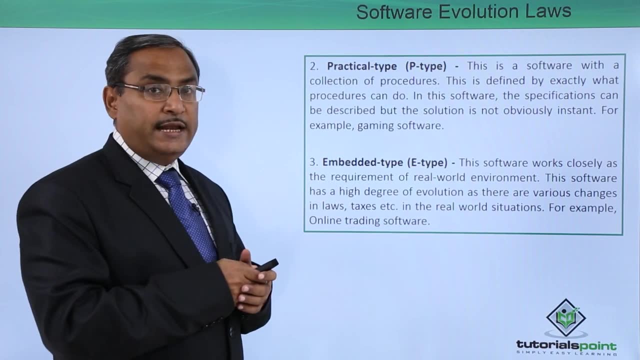 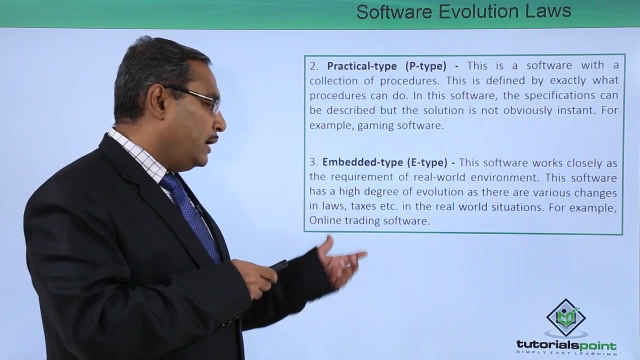 software works closely, as in computer, to software. In software we have essentially key functions as the requirement of real world environment. this software has a high degree of evolution as there are various changes in laws and taxes etc in the real world situations. for example, online trading software should be a good example of embedded type and a type here the multiple.